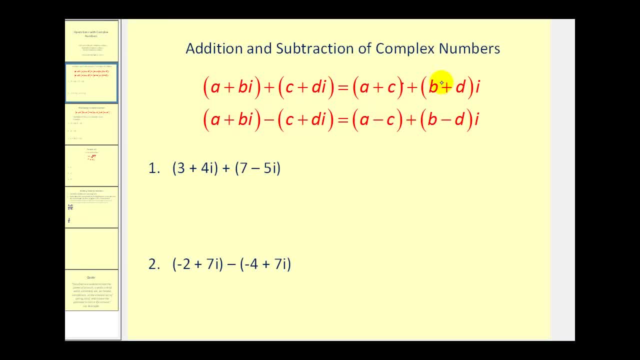 on, But really it's pretty much the same as combining like terms. Each complex number has a real part and an imaginary part. If you're adding two complex numbers, you add the real parts together and then you add the imaginary parts together, And if we have a difference of complex numbers, we find the difference. 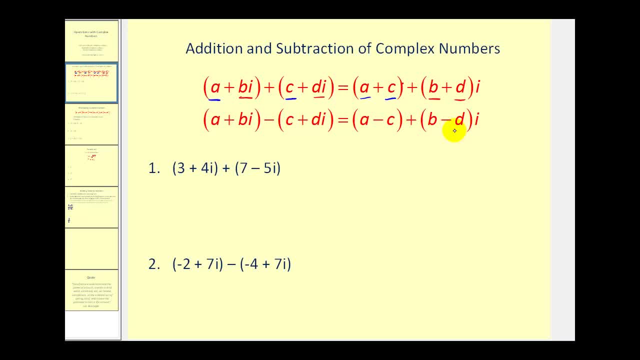 of the real parts and the difference of the imaginary parts. So if we take a look at number one, three plus four, i plus seven minus five, i, Three and seven are the real parts and four, i and negative five, i are the imaginary parts. 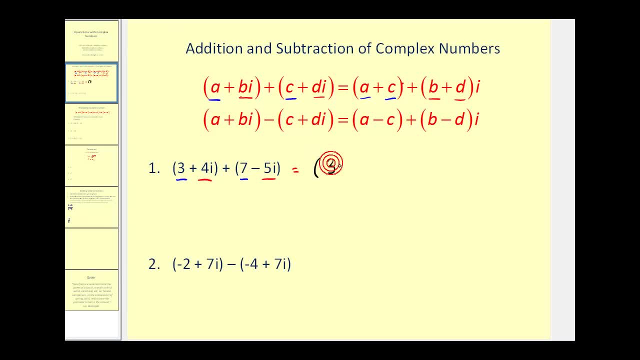 What that means is we can add three plus seven or the real parts, and we can also add four i plus negative five i. The result will be ten plus four i plus negative five i. would be negative one i or negative i, But this is only written as ten minus i. 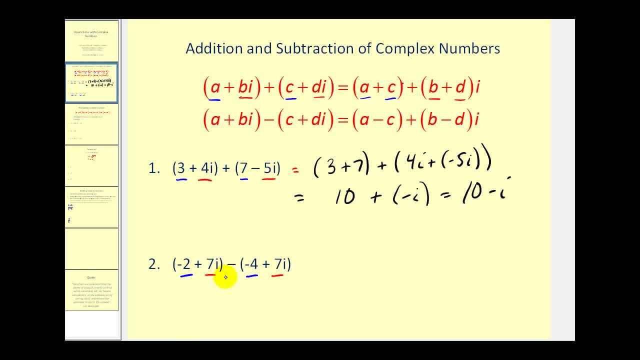 We'll follow a similar process for subtraction. Since we're subtracting now, we'll subtract the real parts and subtract the imaginary parts. So we'll have negative two minus negative four plus seven i minus a positive seven i. So the result: negative two minus negative four. 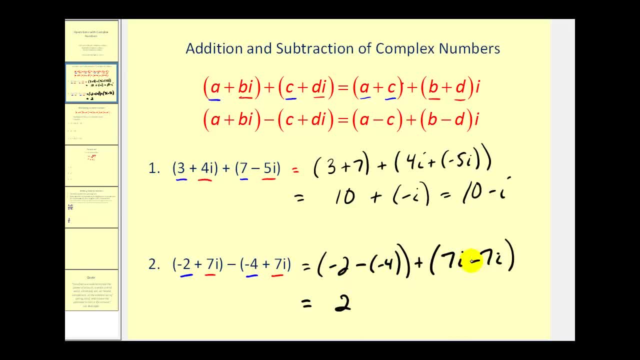 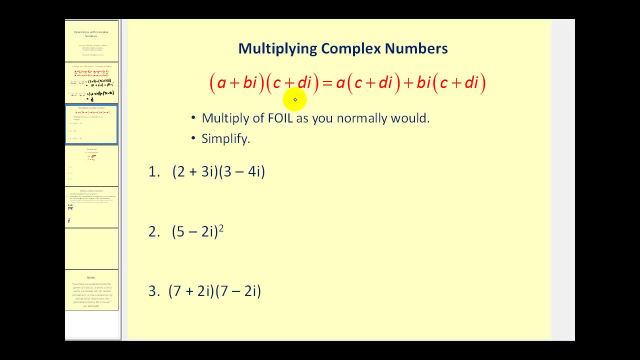 becomes negative, two plus four, or positive, two plus zero, i, which is just zero, so the result is two. So, as you can see, it's pretty much just like combining like terms. Now let's talk about multiplying complex numbers. We will multiply complex. 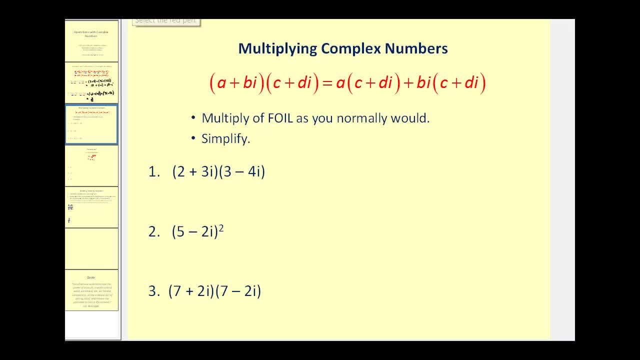 numbers, just like we would multiply two binomials together. We'll multiply a times the quantity c plus d i. Then we'll multiply b i times the quantity c plus d i. Then we'll combine like terms and simplify. So let's go ahead and give it a try Here. we'd have: 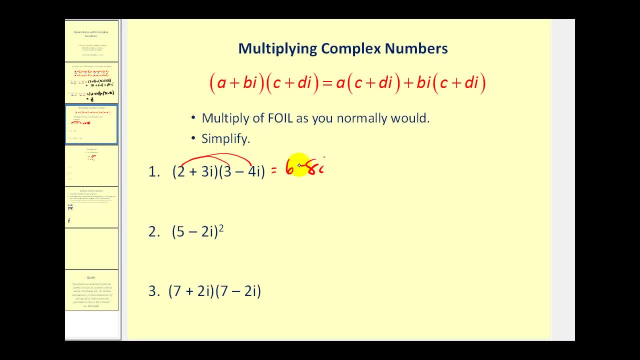 six minus eight i, Then we'd have nine, i minus twelve, i squared. Now remember, a complex number is the form of a plus b i. So we can't leave i squared in this product. So we'll place i squared with negative one, So we'll have negative twelve times negative one. 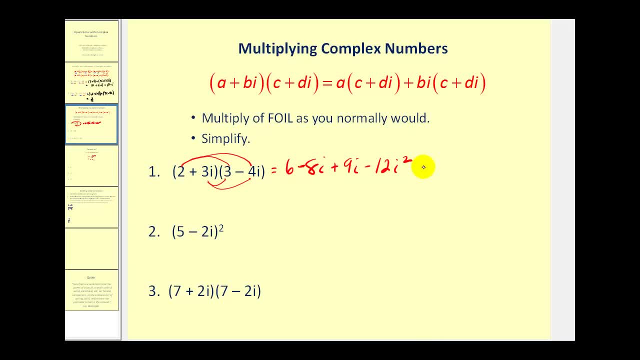 That'll be positive twelve, Then we have a positive six, So that'll give us eighteen, And then we have a negative eight. i plus nine. i would give us a positive one, i, or just plus i. On number two, there's no shortcuts. We have to write this out as: 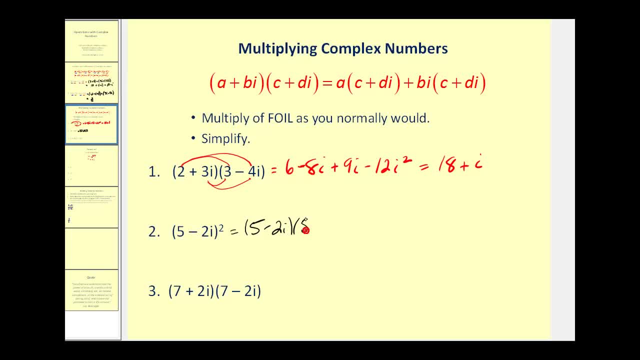 five minus two. i times five minus two. i Go ahead and multiply as we normally would, So we'll have twenty-five minus ten. i minus ten, i again, And then, lastly, we're going to have negative two. i times negative two. i will be positive four. i squared. 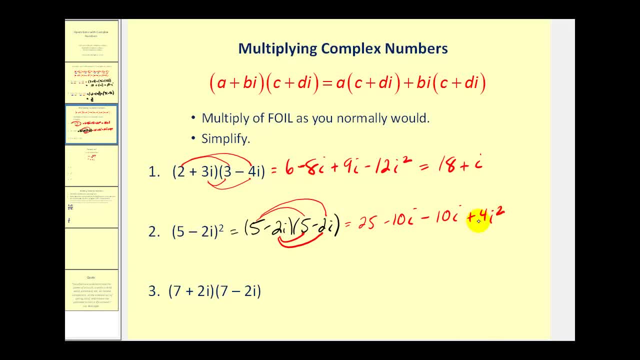 Well, again i squared is equal to negative one. So four times negative one is negative four. Combining negative four with twenty-five will have twenty-one. Combining negative ten: i minus ten, i will be minus twenty i. Now, this last product is a special product. It's called the product of complex conjugates. Notice: 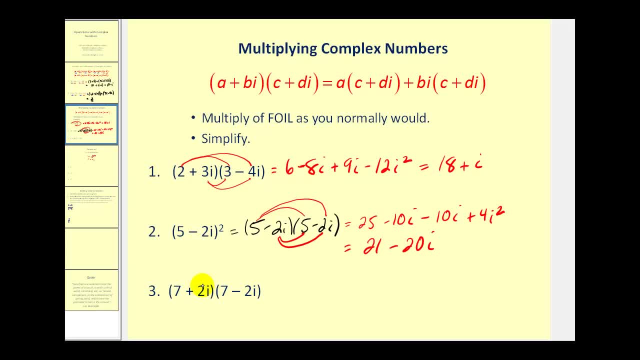 the terms are the same. One's a sum and one's a difference. We have seven plus two i and seven minus two i. The product of these two complex numbers should be real. Seven times seven is forty-nine. Seven times negative two i is minus fourteen i. Two i times seven plus fourteen i And. 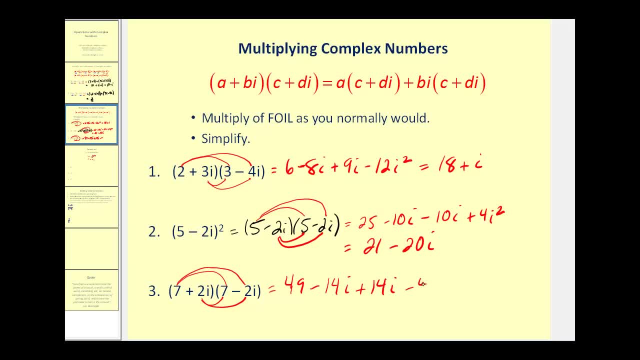 then, lastly, we have negative four i squared. And what's special here is that the imaginary parts of these complex numbers are opposites. So these have a sum of zero. I squared is negative one, So negative four times negative. one is positive. four plus forty-nine is equal. 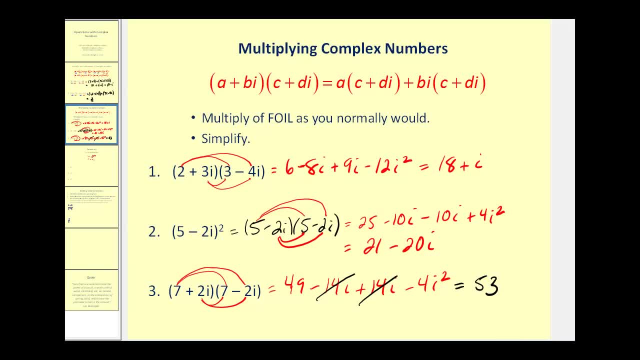 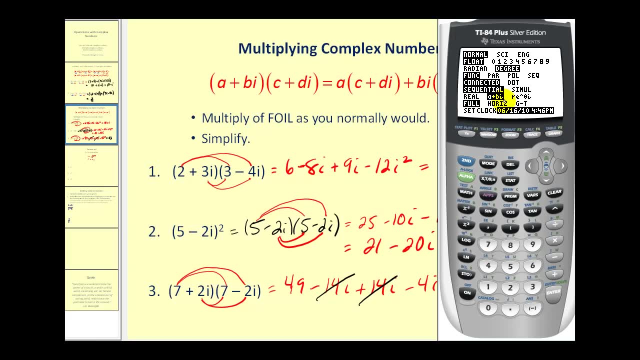 to fifty-three. Now let's go ahead and check these on the graphing calculator. If we press the mode key and you scroll down to here, make sure you have a plus bi selected. That way the calculator will recognize complex numbers. Go back to the home screen and we'll check. 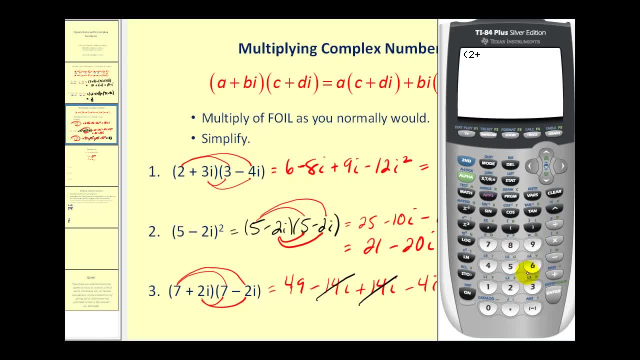 one, two and three. Two plus three i i is located by pressing second decimal. Eighteen plus i is what we had for number one. Let's go ahead and check number two. We have the quantity five minus two i squared, And. 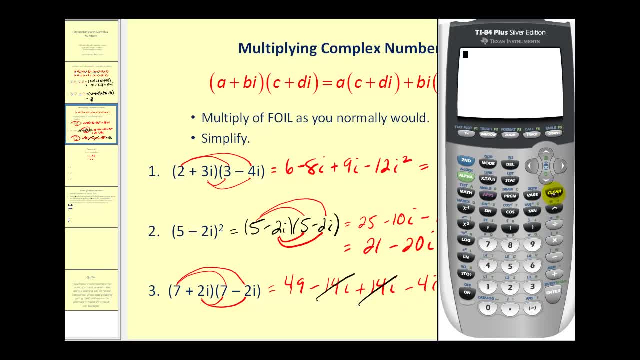 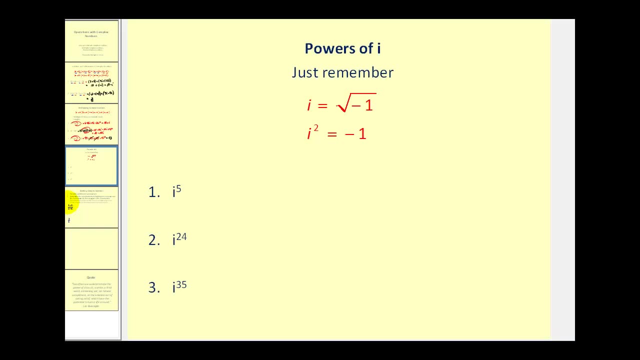 that checks. And the last one, we had fifty-three. Let's check that. We had seven plus two i times seven minus two i, And that checks as well. Let's now talk about powers of i. Now some textbooks talk about dividing by four. I'm going to go ahead and do that. I'm going. 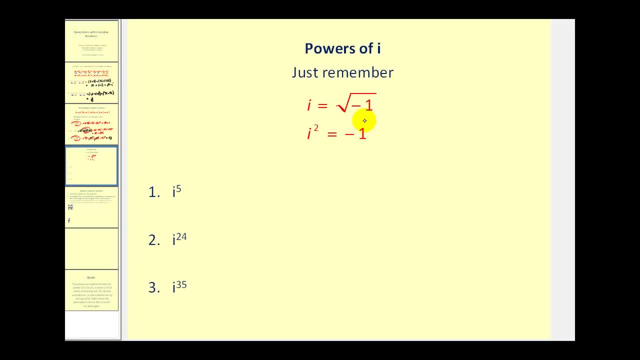 to divide by four, and then there's four different cases, But to me, as long as you can remember that i squared is equal to negative one, you should be able to figure out logically what all these are equal to. This is what I mean by that. We want to determine how many i squareds. 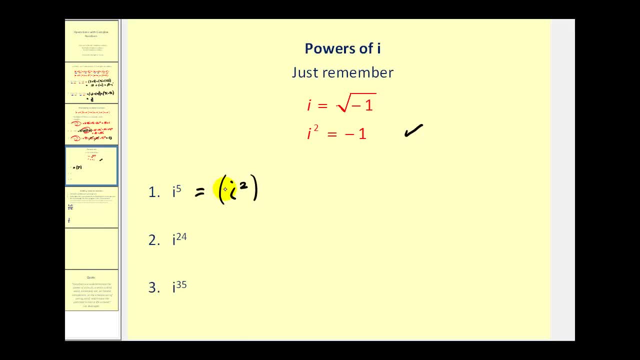 are in i to the fifth. Well, one way to think of that is: how many twos are in five. Well, there are two twos in five. Two times two would be four, With one extra factor of i. Now we'll just replace i squared with negative one. 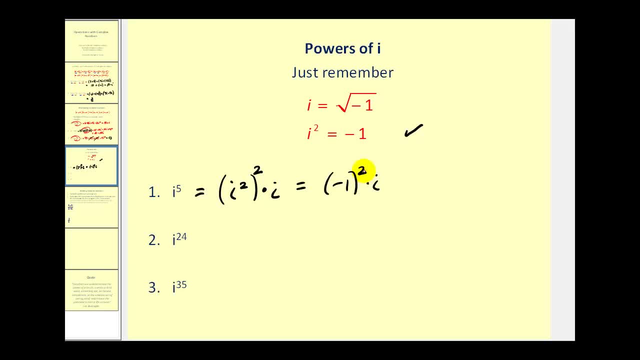 Negative one squared is positive one times i. So the result is i. If i is raised to an odd power, the result will always be i or negative i. Let's take a look at number two. How many i squareds are in i to the twenty-fourth power? Or how many twos are in twenty-four? 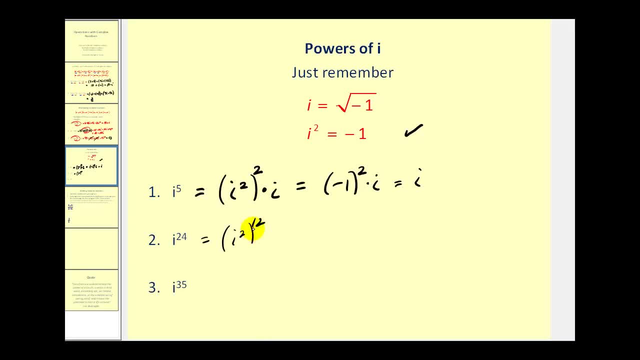 There's twelve twos in twenty-four. This is the same as i. to the twenty-fourth, We now replace i squared with negative one, Negative one. to the twelfth power is positive one. So if we have i raised to an even power, 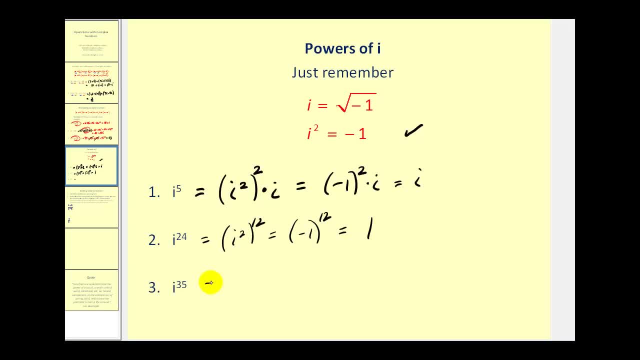 it will always be either one or negative one. Let's go ahead and try one more. How many i squareds are in? i to the thirty-fifth. If we raise this to the seventeenth power, that would be i to the thirty-fourth, with an extra factor of i. Now we have negative one to the. 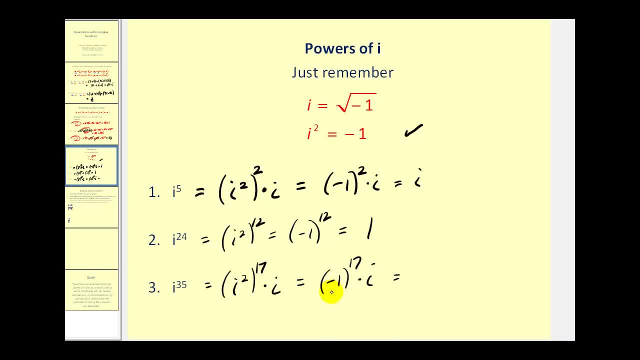 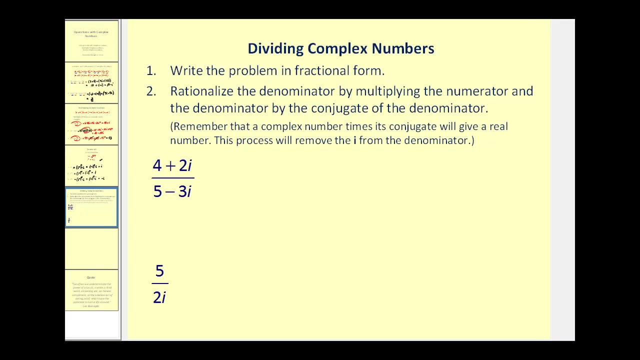 seventeenth power times i. Well, the negative number raised to an odd power will always be negative. So we have negative one times i or negative i. Let's go ahead and finish by talking about the division of complex numbers. We will first write the problem in fractional form, and then we will rationalize the denominator by 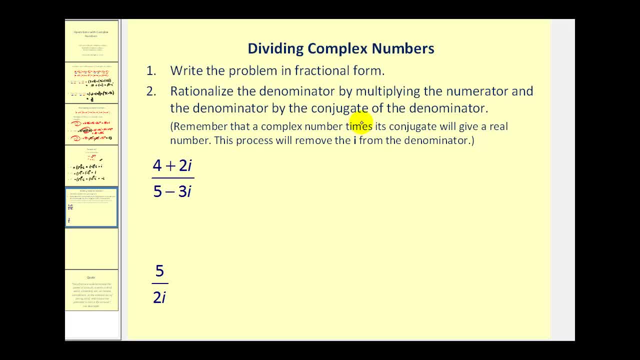 multiplying the numerator and denominator by the conjugate of the denominator. In order to divide these two complex numbers, we must multiply by the conjugate of the denominator in both the numerator and denominator. So the conjugate of five minus three i is five plus three i. So multiply the numerator. 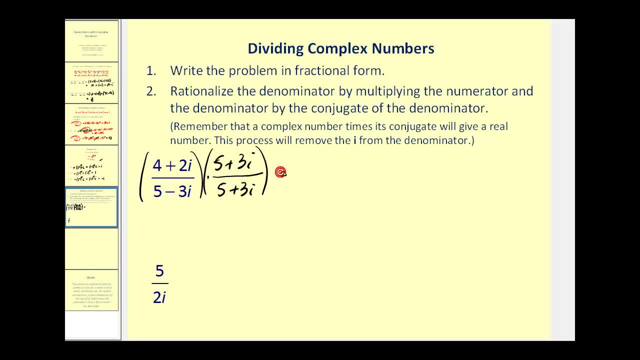 by the same thing. Remember: the product of these conjugates should be a real number. So let's go ahead and multiply the denominator first. Five times five, that would be twenty-five. The next two products should be opposites. Here we have a positive fifteen i and then 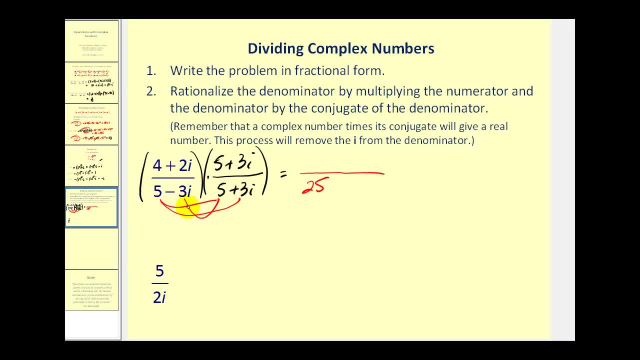 we have a negative fifteen i Those would simplify out- and the last product is negative nine i squared. Now let's go ahead and multiply the numerator. We have twenty plus twelve, i plus ten, i plus six i squared. Let's simplify this. 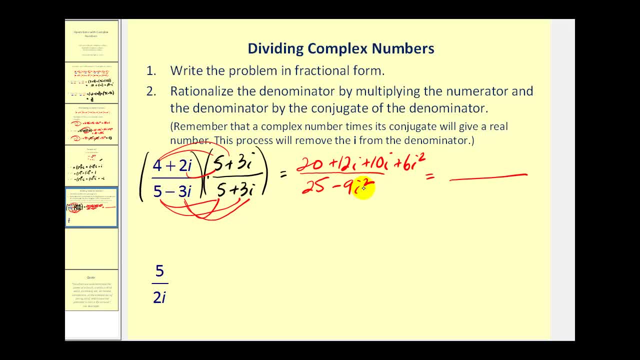 We know that i squared is negative one, so negative nine times negative. one is positive. nine plus twenty-five That would give us thirty-four In the numerator. this would end up being a negative six, since i squared is negative one. So twenty plus negative six would be fourteen, and then twelve. i plus ten, i would be twenty-two. 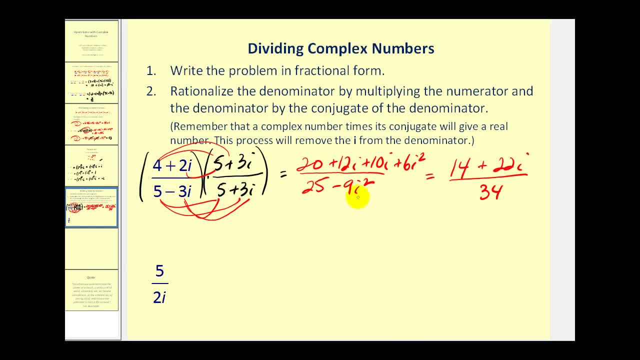 i. Let's write this in a plus b i form and then simplify So we'd have fourteen over thirty-four plus twenty-two over thirty-four i. This simplifies to seven-seventeenths plus eleven-seventeenths i. 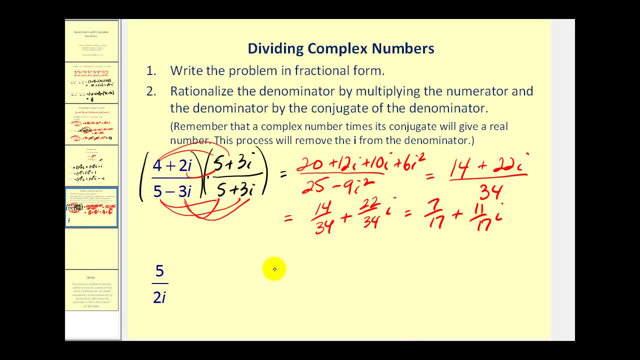 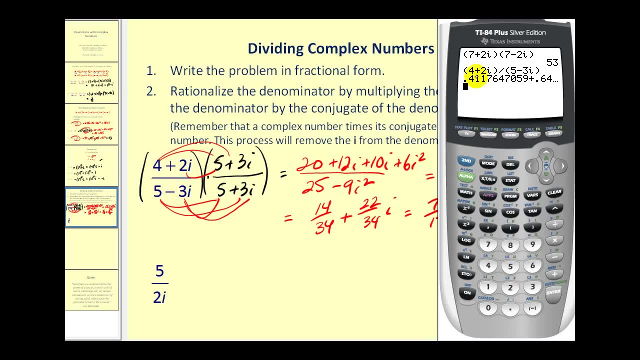 This is a lot of work. Let's go ahead and check. Let's check this one on the calculator. Numerator was four plus two. i. Denominator was five minus three, i. Let's convert this to fraction notation by pressing math enter, enter and we have seven-seventeenths. 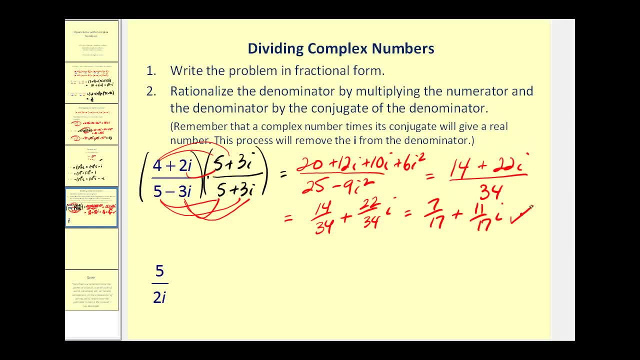 plus eleven-seventeenths i, And that's exactly what we had as well. Okay, on this last problem, our denominator is two i. You can think of two i as zero plus two i. Therefore, the conjugate would be zero minus two i. 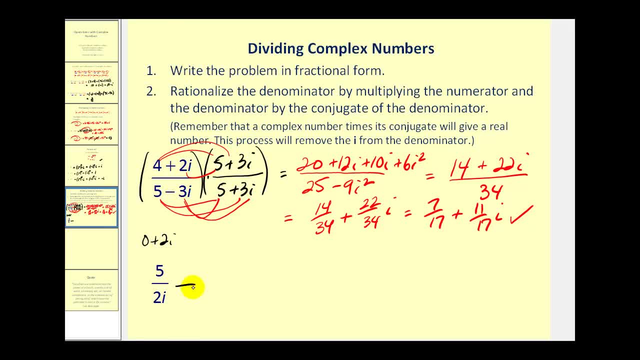 Or just negative two. i So multiply both the numerator and denominator by negative two. i We'll simplify. So our denominator would be negative four, i squared. Our numerator would be negative ten. i Again i squared- is negative one, So negative one times negative four would be positive four over negative ten. i.